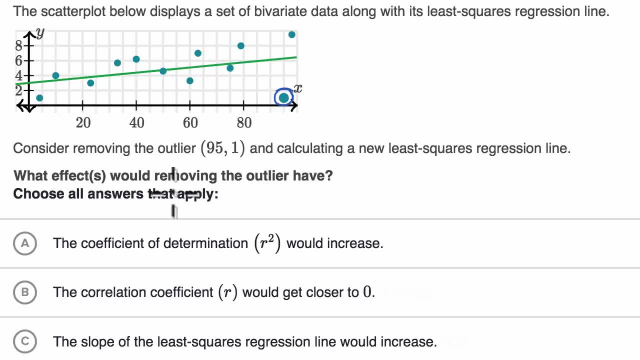 What effects would removing the outlier have? Choose all answers that apply, Like always, pause this video and see if you could figure it out. Well, let's see, even with this outlier here we have an upward sloping regression line, And so it looks like our r already. 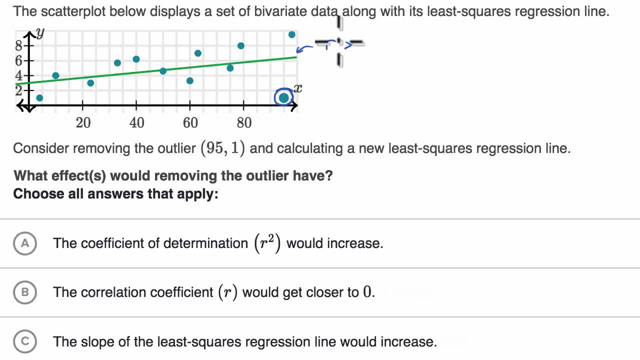 is going to be greater than zero and of course it's going to be less than one. So our r is going to be greater than zero and less than one. We know it's not going to be equal one, because then we would go perfectly through all of the dots. 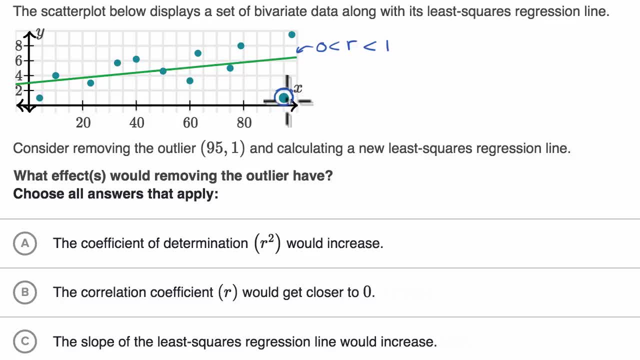 And it's clear that this point right over here is indeed an outlier. The residual between this point and the line is quite high. We have a pretty big distance right over here. It would be a negative residual, And so this point is definitely bringing down the r. 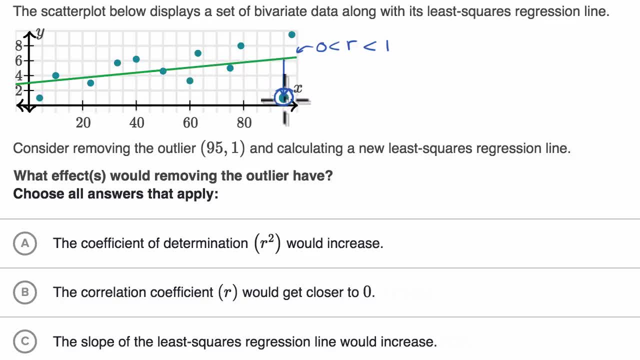 and it's definitely bringing down the slope of the regression line. If we were to remove this point, we're more likely to have a line that looks something like this, in which case it looks like. that looks something like this, in which case it looks like. 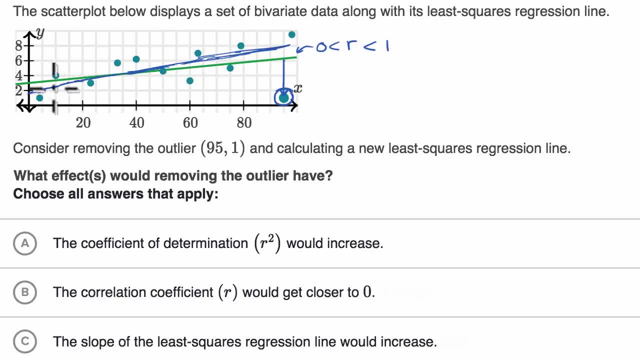 that looks something like this, in which case it looks like we would get a much, a much, much, much better fit. The only reason why the line isn't doing that is it's trying to get close to this point right over here. 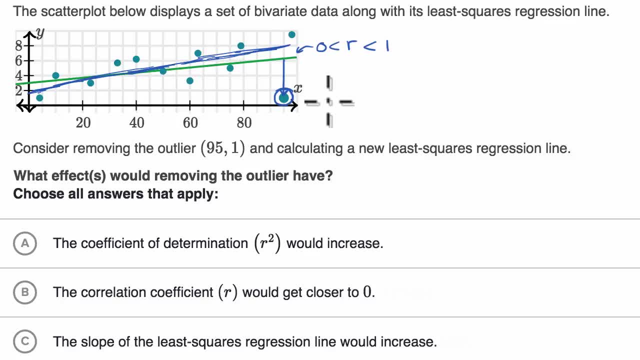 So if we remove this outlier, our r would increase, So r would increase And also the slope of our line would increase And slope would increase. We'd have a better fit to this positively correlated data And we would no longer have this point dragging the slope. 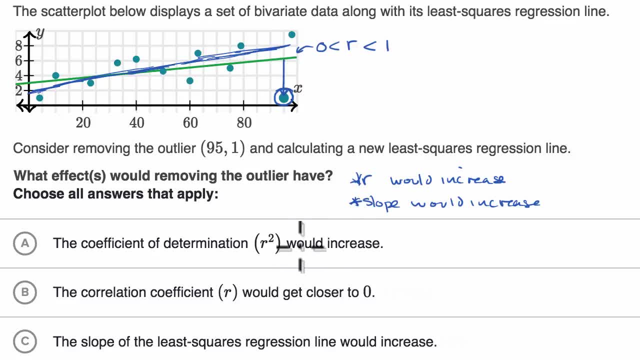 And we would no longer have this point dragging the slope down anymore. So let's see which choices apply. The coefficient of determination, r squared, would increase. Well, if r would increase, then squaring that value would increase as well. So I will circle that. 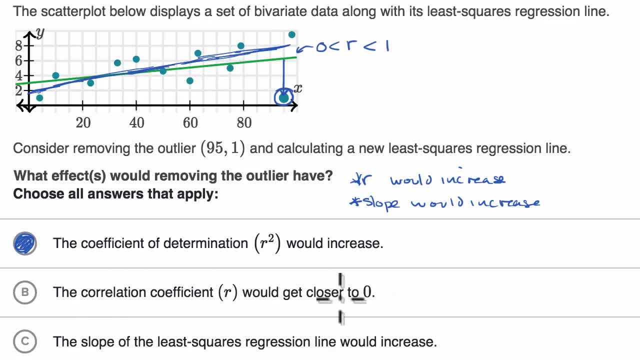 The coefficient, the correlation coefficient r would get close to zero. No, in fact it would get closer to one, because we would have a better fit here, And so I will rule that out. The slope of the least squares regression line would increase. 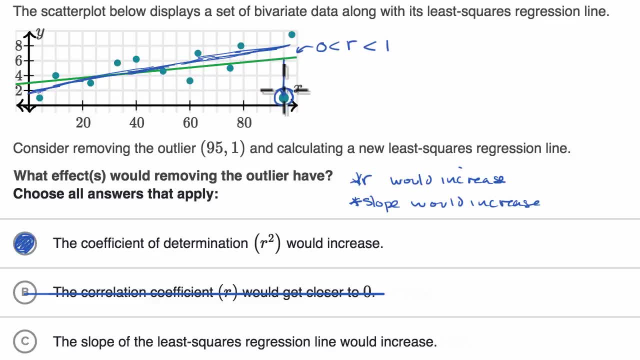 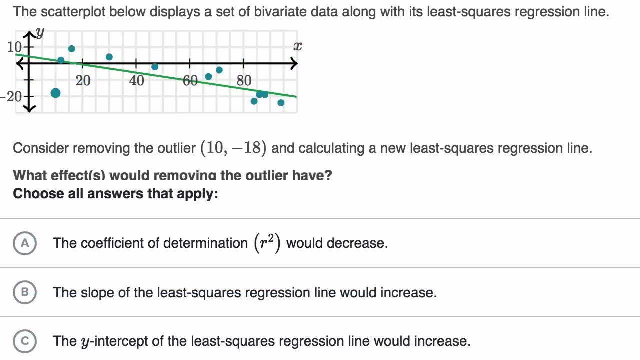 Yes, indeed, this point, this outlier, is pulling it down. If you take it out, it'll allow the slope to increase, So I will circle that as well. Let's do another example. The scatter plot below displays a set of bivariate data. 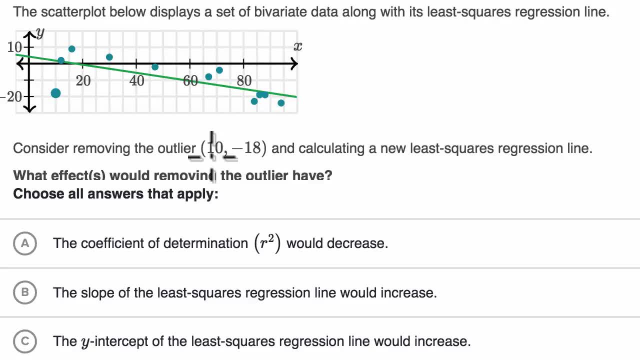 along with its least squares regression line. Same idea: Consider removing the outlier 10 comma, negative 18.. So we're talking about that point there And calculating a new least squares regression line. So what would happen this time? So as is. 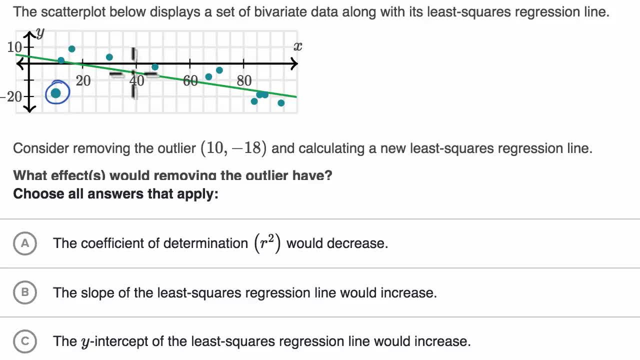 without removing this outlier, we have a negative slope for the regression line. So we're dealing with a negative r. So we already know that negative one is less than r, which is less than zero. without even removing the outlier, We know it's not going to be negative one. 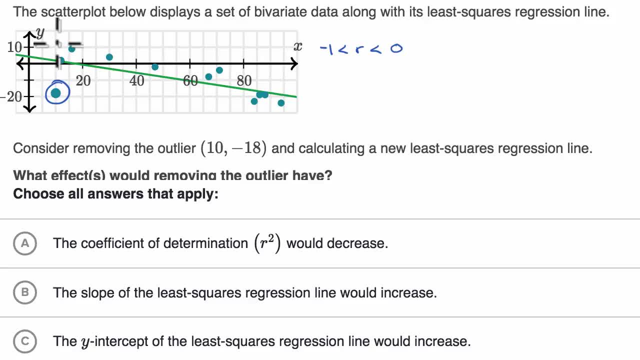 If it was negative, if r was exactly negative one, then it would be a downward sloping line that went exactly through all of the points. But if we remove this point, what's going to happen? Well, the least squares regression is being pulled down here. 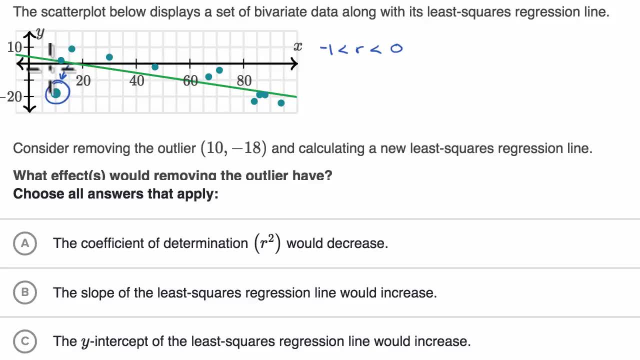 by this outlier. So if you were to remove this point, the least squares regression line could move up on the left-hand side, And so you'll probably have a line that looks more like that- And I'm just hand drawing it. But even what I hand drew looks like a better fit. 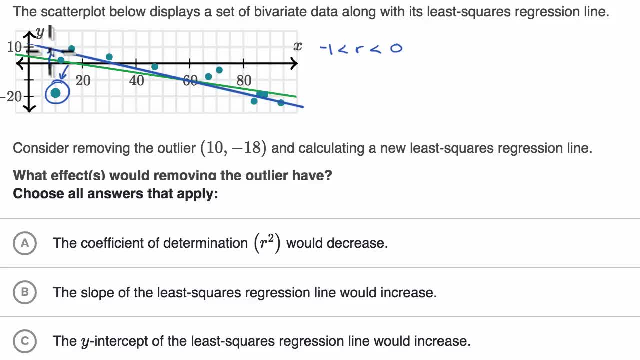 for the leftover points And so clearly the new line that I drew. after removing the outlier, this has a more negative slope. So removing the outlier would decrease r, r would get closer to negative one. It would be closer to being a perfect negative correlation. 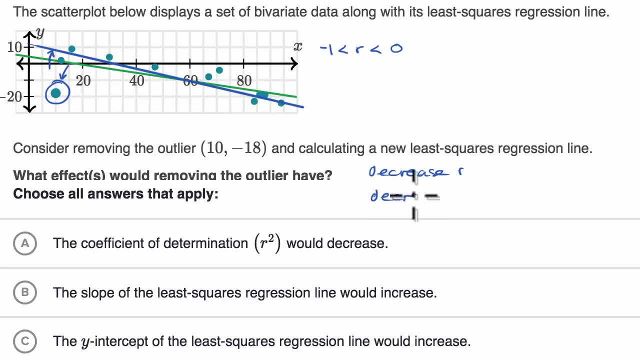 And also it would decrease the slope. Decrease the slope Which choices match that. The coefficient of determination r squared would decrease. So let's be very careful. r was already negative. If we decrease it it's going to become more negative. 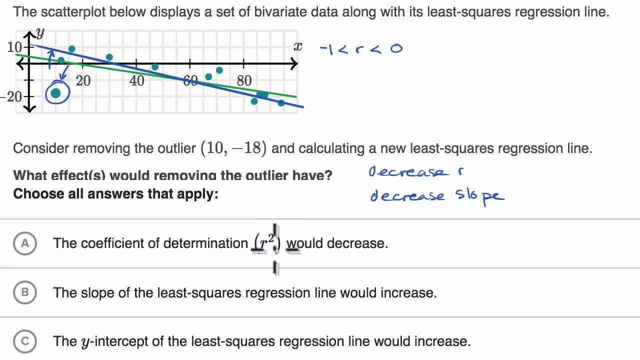 If you square something that is more negative, it's not going to become smaller. Let's say: before you remove the data, point r was. I'm just going to make up a value. Let's say it was negative 0.4..